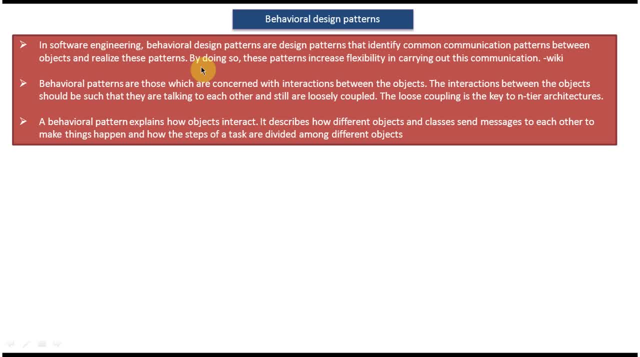 So that is what this behavioral design patterns talk about. And next explanation: Behavioral patterns are those which are concerned with interaction between the objects. The interaction between the objects is called behavior pattern. The interaction between the objects should be such that they are talking to each other and still are loosely coupled. 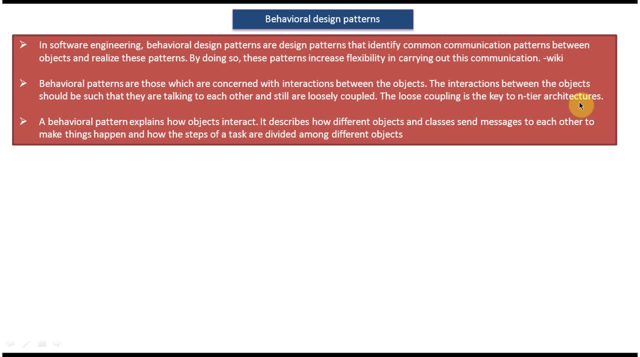 The loose coupling is the key to entire architecture. So this behavioral design pattern is concerned with interaction between the objects. And interaction between the objects should happen and it should talk to each other, But the two objects should be loosely coupled. So loosely coupled is the key factor in the entire architecture. 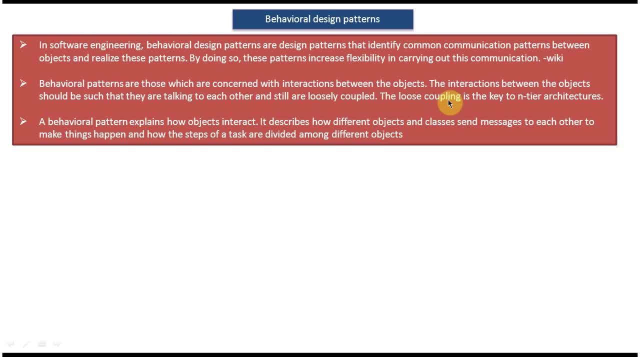 So it should be loosely coupled. And third definition is a behavioral pattern. explains how objects interact. It describes how different objects and classes send message to each other to make things happen and how the steps of task are divided among different objects. So basically, this behavioral design pattern explain how two objects are interact. 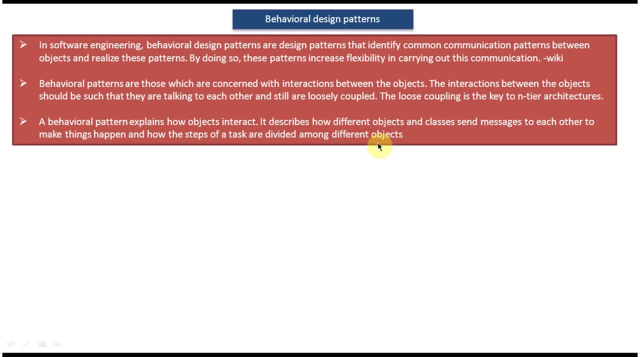 It describes how objects or classes are sending messages to talk to each other in order to accomplish some functionality. And next I will cover what and all patterns which will come under the behavioral design patterns. So this many patterns which will come under the behavioral design patterns. 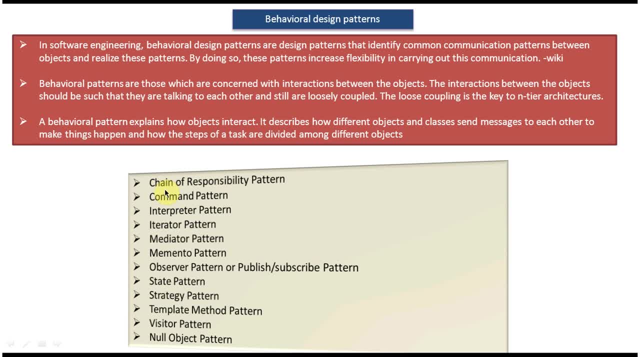 I will read out one by one. First one is chain of responsibility pattern: Command pattern, Interpreter pattern, Iterator pattern, Mediator pattern, Momento pattern, Observer pattern Or publish or subscribe pattern. So another name of observer pattern is publish or subscribe pattern. 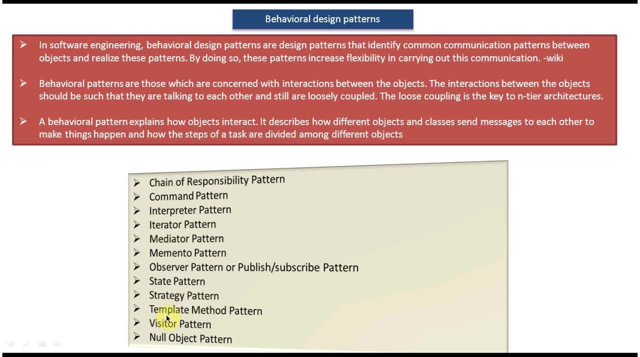 And state pattern, Strategy pattern, Template method pattern, Visitor pattern And null object pattern. So this many patterns which will come under the behavioral design patterns. I have created videos for each and every pattern and where I have explained what is the definition of each and every pattern.